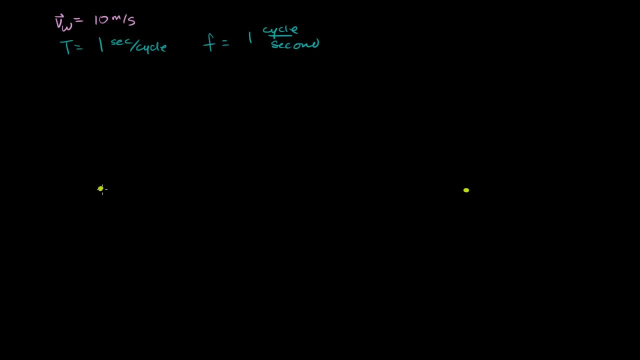 Where is that crest going to be? now Let's think about the stationary character. Well, in this guy it emitted the crest 1 second ago. It's moving outward. So this is outward. It's moving outward radially. I need to give a direction if I'm giving a vector quantity. So it's moving outward at 10 meters per second. So if it emitted it 1 second ago, it's going to be 10 meters radially outward from the source. So maybe that is right over there. Let me draw it a little bit neater like that. 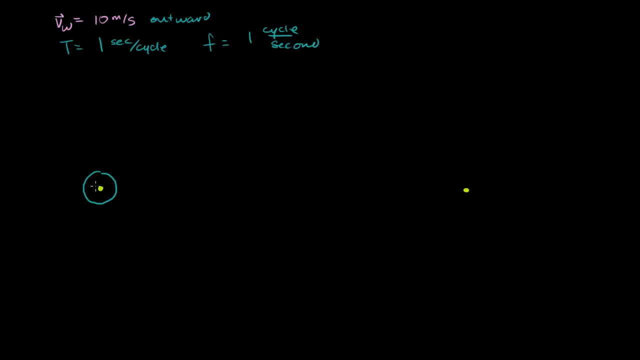 A little bit neater. That's pretty good. So that's where that crest will be. Now, what about this guy? Where is the crest that this guy emitted 1 second ago? Well, you might want to just draw a radius 10 meters around this guy as well, but he wasn't here 1 second ago. He was 5 meters to the left. Remember, he's moving 5 meters per second to the right, So 1 second ago he was 5 meters to the left. So maybe that places him right over there. 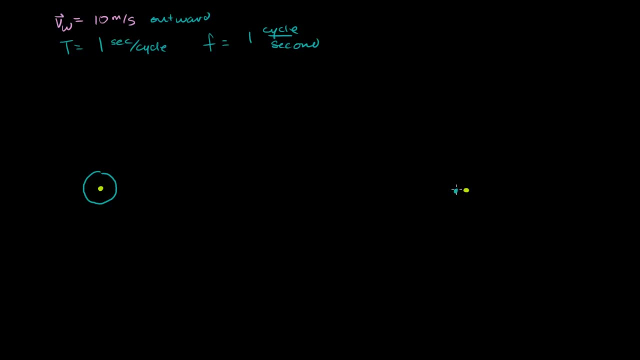 The crest that he emitted 1 second ago isn't going to be 10 meters from this guy. It's going to be 10 meters radially outward from that guy. So let me just copy and paste this right here. So copy and paste and just put it right over there. So this is where he is now. That's where he was 1 second ago, where he emitted this crest that has now traveled 10 meters away. This is a little inexact, so I can draw it a little bit like that. 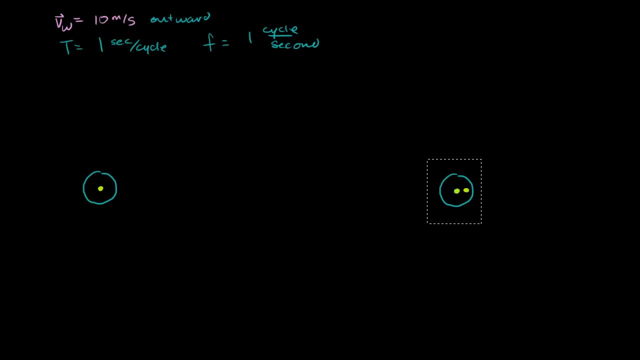 5 meters. that's 10 meters away. But you get the general idea. Now let's keep going. Let's think about the crest that both of these guys emitted 2 seconds ago, So this guy has been stationary the whole time. If he emitted it 2 seconds ago, it's traveling at 10 meters per second. It's going to be 20 meters radially outward from the center, from the source, So it will look something like that. 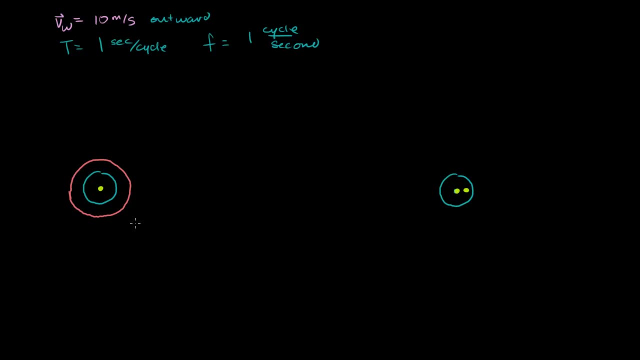 I'm just drawing the crests of the waves. If you think of water, a pebble being dropped into a pond, these are just the high points on the wave that spreads radially outward from where the pebble was dropped. Now this guy- once again, you can't just draw a circle around this- because he wasn't here 2 seconds ago. He was right here. He was right here 2 seconds ago. 1 second ago he was 5 meters to the left. A second before that he was 5 meters more to the left. So that wave that he emitted then is going to be 20 meters. 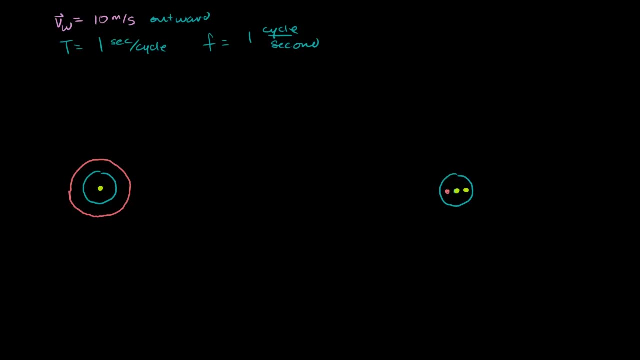 radially outward from this point, And so let me just copy and paste this right here. So copy and paste. So the center isn't going to be that or that, It's going to be that point where he was 2 seconds ago. Let's do this again. Let's do it again. Let me use pink. So what about the crest that either of these sources emitted 3 seconds ago? Well, it would be 30 meters radially outward. So another 10 meters. 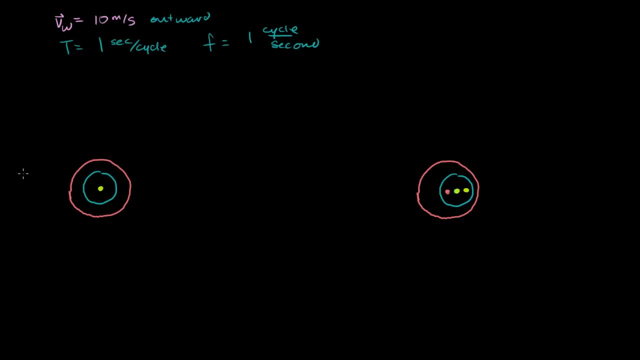 So it will be out here. It will be out there, Just like that. This guy's been stationary the whole time. But what about this guy? Well, he wasn't here 3 seconds ago. He was here 1 second ago, here, 2 seconds ago, there, 3 seconds ago there. So we're going to be 30 meters radially outward from this point. So once again, I can just copy and paste this right here. 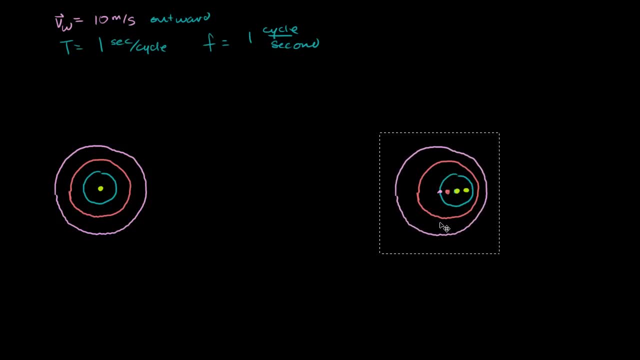 So copy and paste And it should be centered around that point, Around that point right there. Now let's think a little bit about what the perceived frequency of this wave would be for a couple of observers. So we could put an observer here, really anywhere around this guy. We could put an observer right here, And then we could put another observer right here. Now, what's this guy going to perceive? 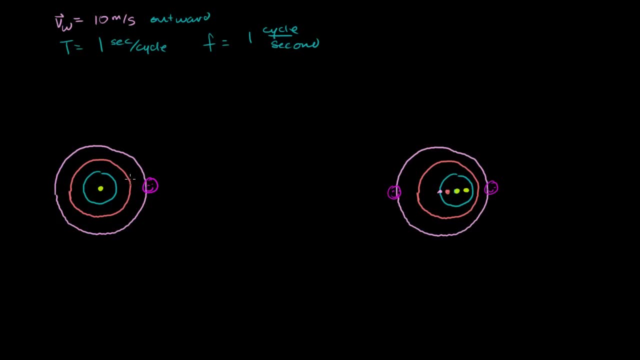 Second, he's getting a pulse being. Well, there's a couple of things to think about. First of all, what is the wavelength of at least this wave right here? Well, every second he's emitting a pulse. So a second ago the pulses out there would have traveled 10 meters. And then he emits another pulse. So the pulses are going to be 1 second apart, But since they travel 10 meters in that 1 second, they're also going to be 10 meters apart. So the wavelength in this case is going to be 10 meters. The distance between these crests are 10 meters. 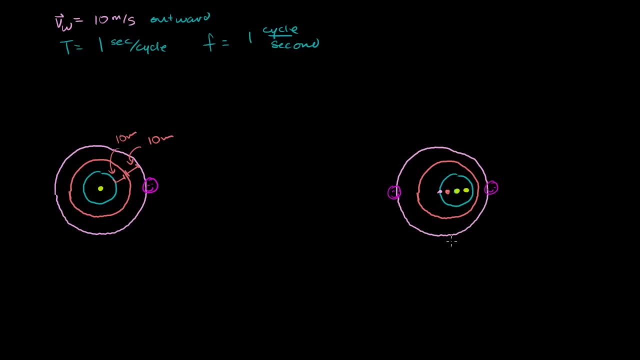 Now, what about this situation right here? Well, it depends on kind of what side, whether the source is coming towards you or whether it's going away from you. That's the situation with this guy. When it's moving towards you, it's emitting a pulse. So let's say it emitted a pulse right here, And then it moves 5 meters to the right before emitting the next pulse. So instead of them being 10 meters apart, in this case, this guy has kind of closed the distance by 5 meters over here. 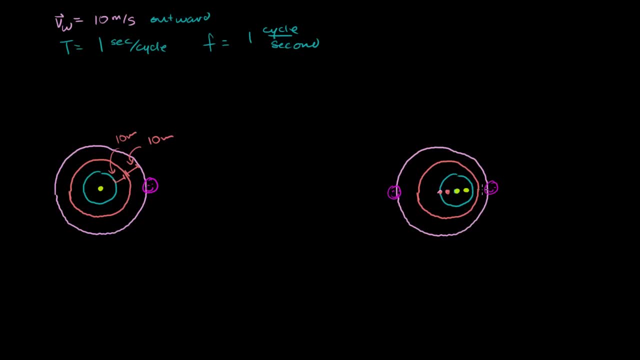 These pulses are only going to be 5 meters apart. So over here the wavelength is only 5 meters And you can see it visually. This distance right here is half of this distance. These are 5 meters apart, And on the left-hand side, if you're on the side of the source that the source is moving away from, it would be 10 meters, But every second the source is also moving 5 more meters away from you. So this wavelength right here, this perceived wavelength right here, 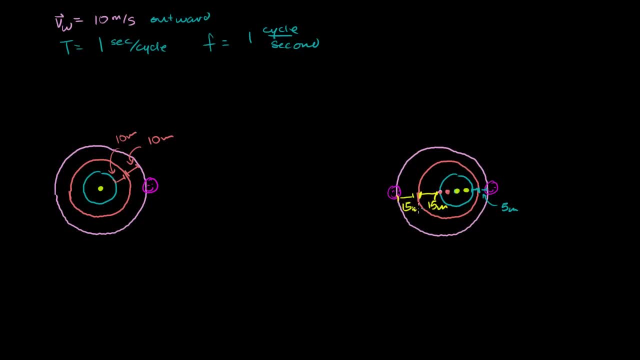 is 15 meters And we can see it visually. That's the whole reason why I drew it this way. Now, what's going to be the perceived frequencies for this? Well, this guy, you know he has one crest passing him right now. It's going to take exactly one second for the next crest to get to him, because it's traveling at 10 meters per second. So he is going to perceive one crest, or one cycle per second, or a frequency of 1 hertz, which makes sense. This is stationary. They're both stationary relative. 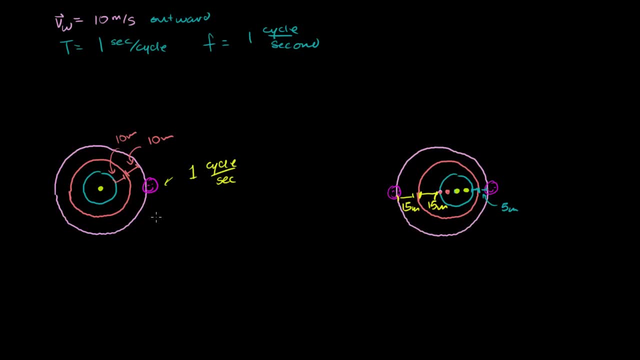 They're relative to each other And we're also talking about classical physics. We're not getting into relativity and all of that, But the observed frequency is the exact frequency that was emitted by this guy right there. Now, what about this situation? Well, each of these crests are 5 meters apart for this guy. If you imagine that this was some type of a train coming towards this guy. each of these crests are only 5 meters apart, But they're traveling at 10 meters per second. So how many crests are you going to see in a 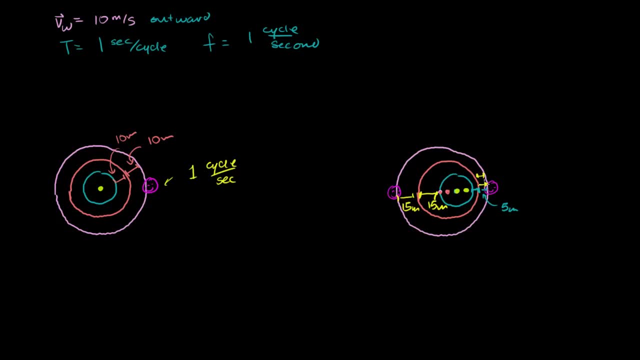 second. Well, you're going to see two of them: This one's going to take half a second to reach you, And then the next half a second this one's going to get to you. Or you could say: this one takes half a second to reach you, Then this one's going to take one second to reach you. So there's two ways to think about it. You could say your period in this situation is 1 half of a second per cycle, Or you could invert it And you could say that the observed frequency is going to be two cycles per second. 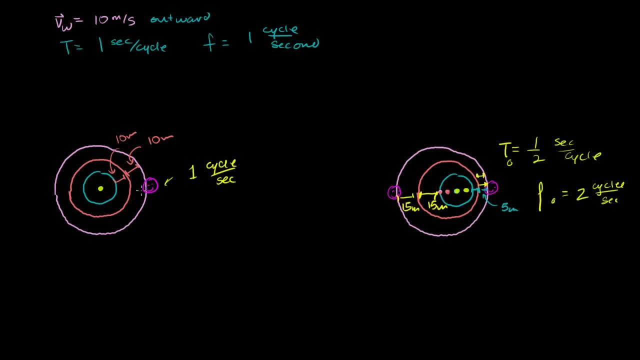 And already notice. this guy's experiencing a higher frequency than this guy over here because these wave fronts or these crests are just passing by him more frequently. Because this guy's moving in the same direction as this guy. they're closer together. Now this guy's going to experience the opposite thing. Let's say that this crest is just passing him by. How long will it take for the next crest to cover that 15 meters? Well, they're going at 10 meters per second. It's going to be 1.5 seconds. 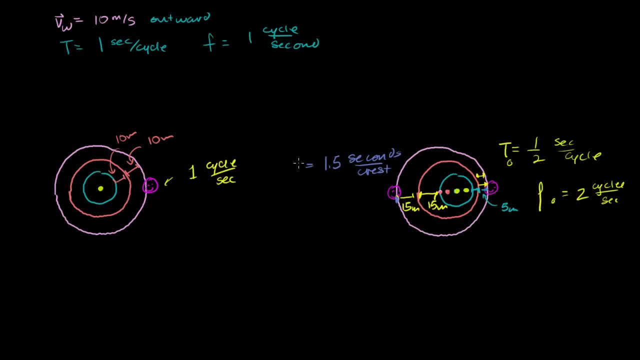 Seconds per crest. That's going to be the observed period for this guy. And if you take the inverse of that, that's 1.5 is 3 halves, That's 2 thirds of a- or you could say- crest, or 2 thirds of a- cycle per second. So when the source is moving away from this observer, the frequency, or the perceived frequency, is lower than the frequency of the actual emitted wave.